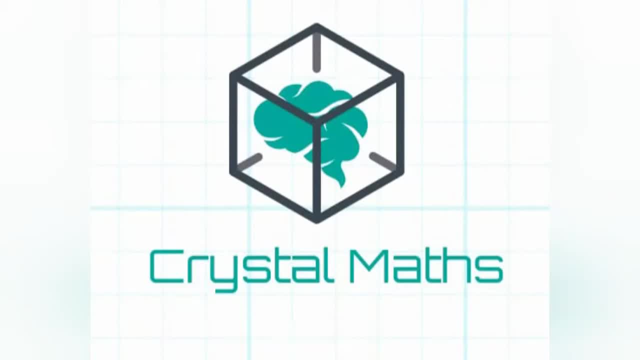 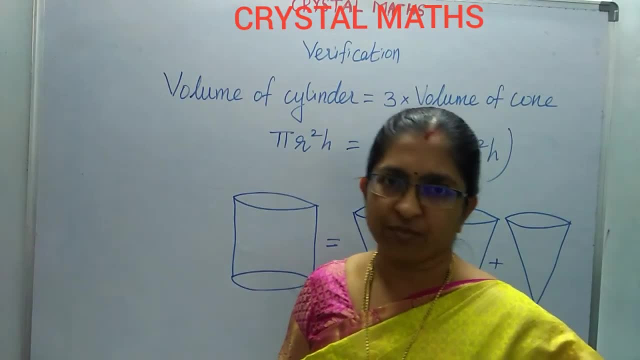 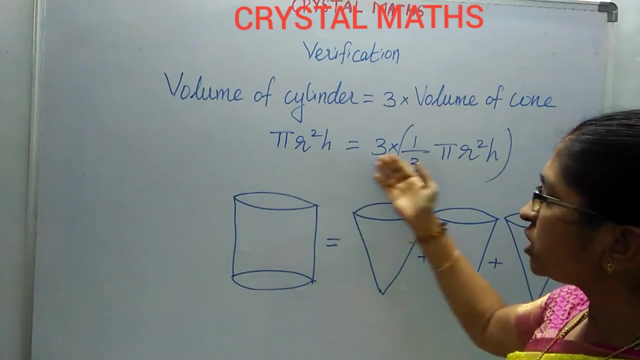 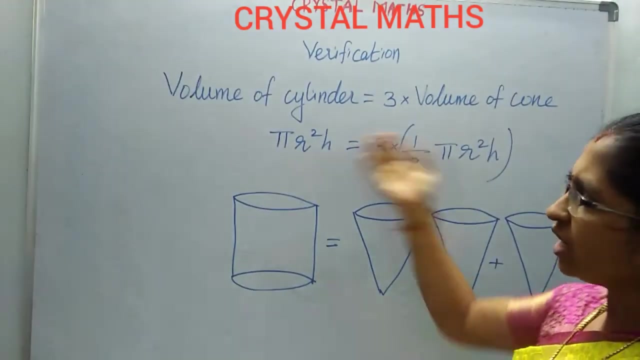 Namaste, welcome to crystal maths. Today we are going to see one small activity. We know that one volume of cylinder equal to three times the volume of cone. So pi r square h is equal to 3 into 1 by 3 pi r square h By formula. maybe we can identify very clearly. 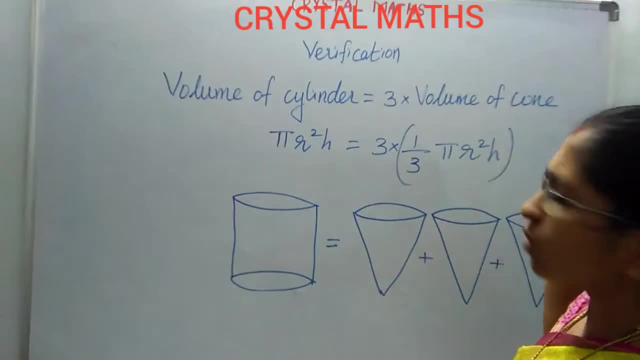 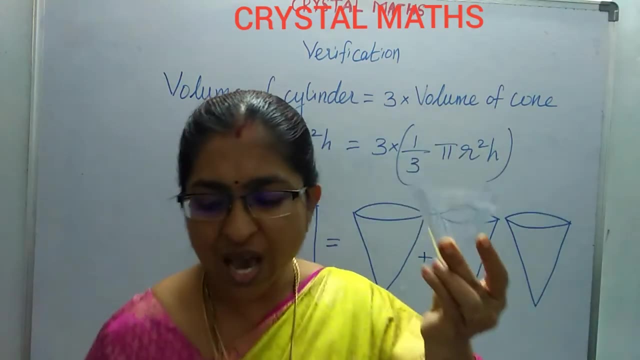 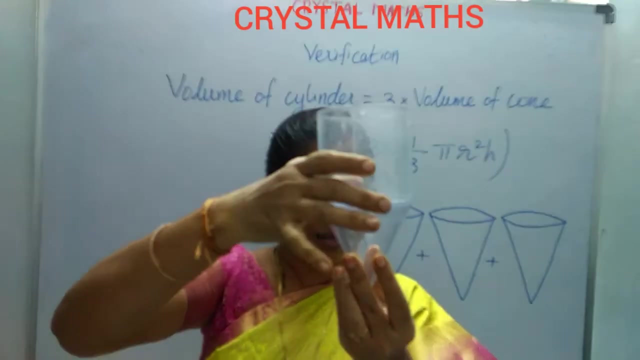 this is. that is, volume of cylinder is three times the volume of cone. Now we are going to verify that one. I am taking the cone over here as well. one cylinder, The both are in the same base. That means the radius of the both- the cone as well as cylinder- is same. 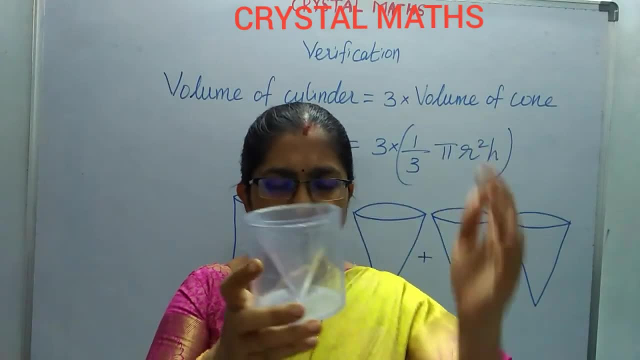 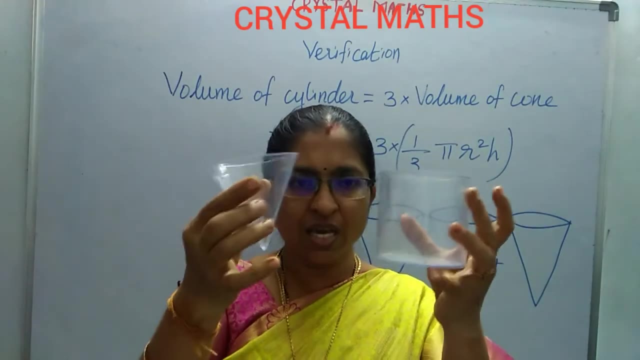 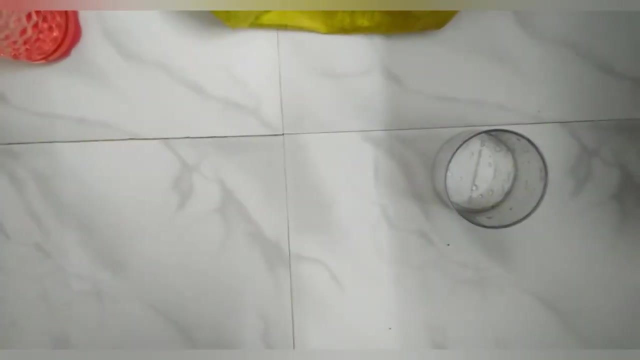 base, Even if I am flipping inside also, it is exactly fitting over there. Now, if both are inside Same radius and same height, the volume of cone will be equal to one third volume of cylinder. Come, let us verify the activity. I am taking one cone, That is cone I am filling. 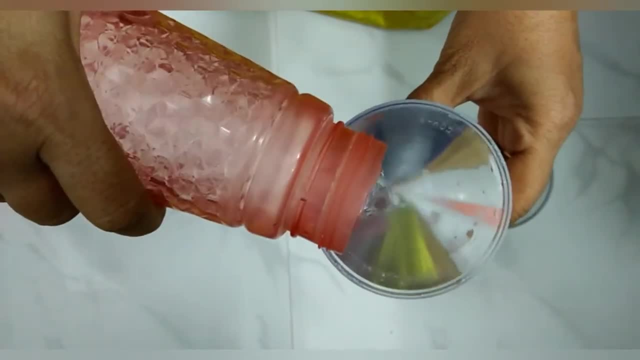 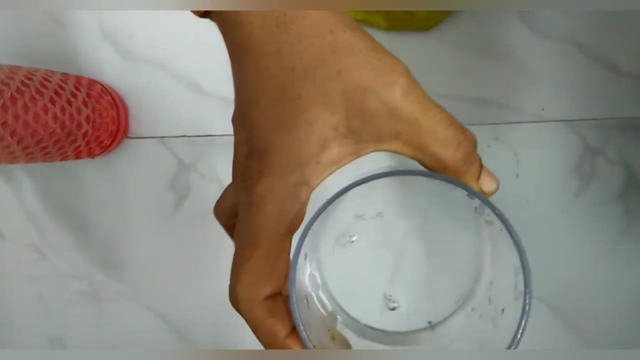 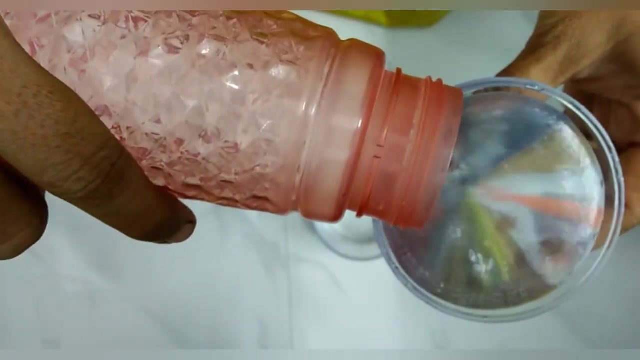 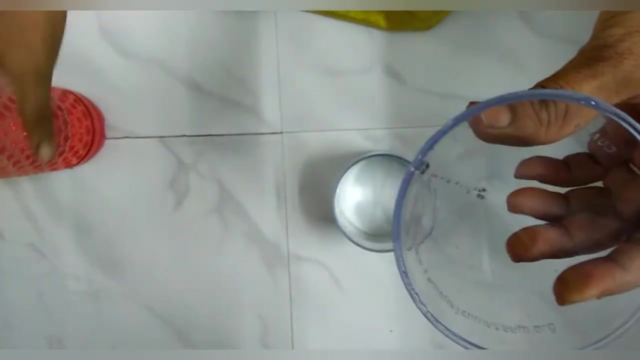 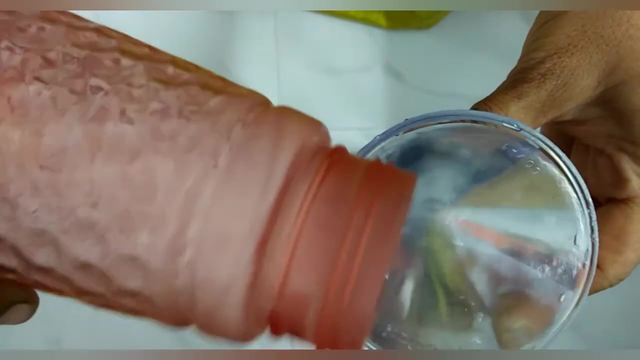 the water completely and I am going to fill it in cylinder One time, Second time And third time. if it is exact, we can identify that it will be equal to three times To the rim. I fill the water, Oh, One time. 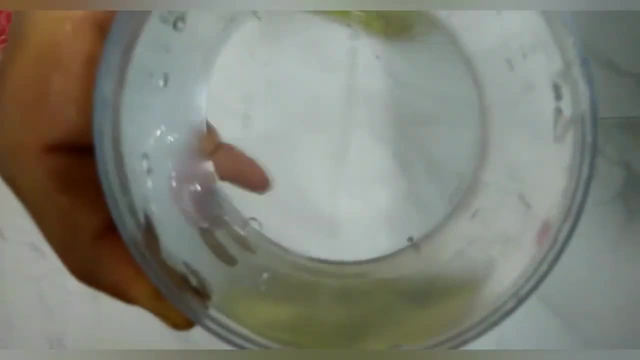 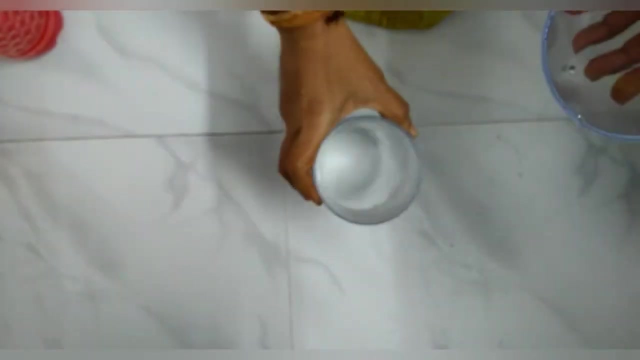 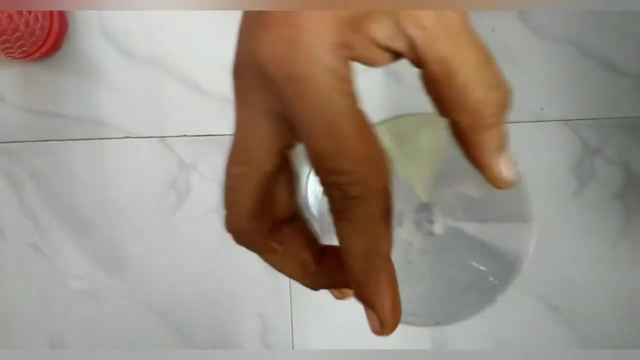 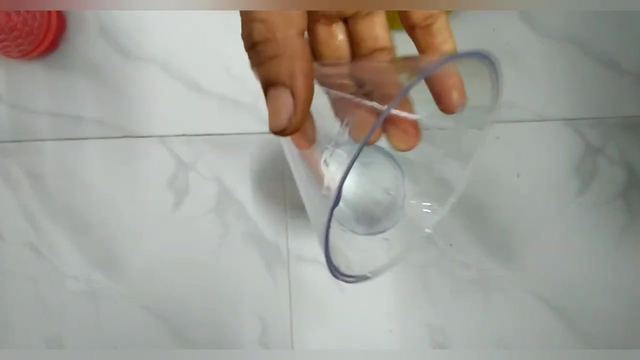 Two times, Three times, Three times, So it is completely. water is complete till the rim of the cylinder. So from this we can refer that volume of cone will be equal to one third the volume of cylinder. Or we can say in opposite also: volume of cylinder equal to three times the volume of cone. Thank you, Thanks, Thanks.